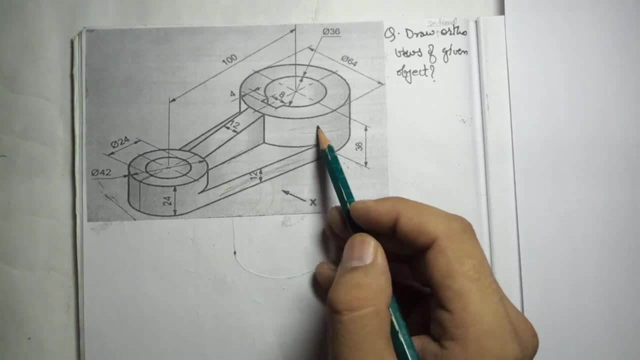 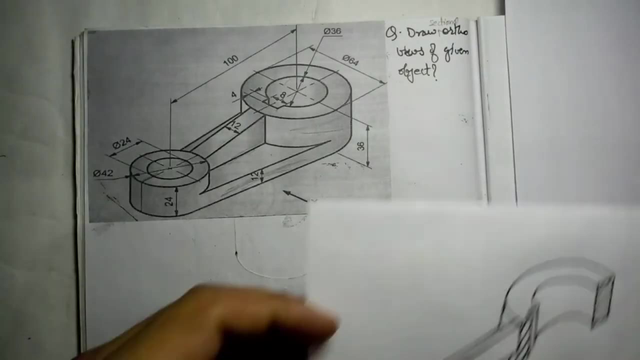 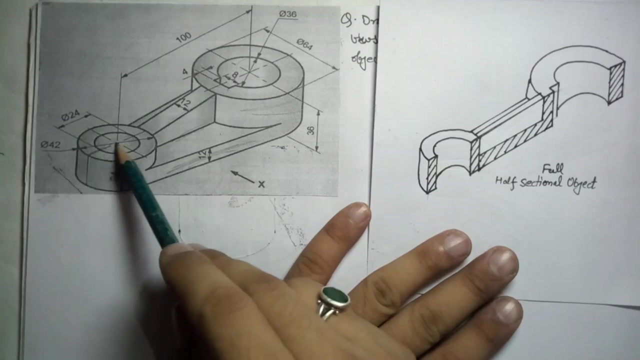 Draw the normal orthography, convert the hidden line into object line. then you have to draw section line with hatching. So just to make it more clear, I have drawn one sectional. object means if I have to cut we have to do the full sectioning means we have to cut fully the object. 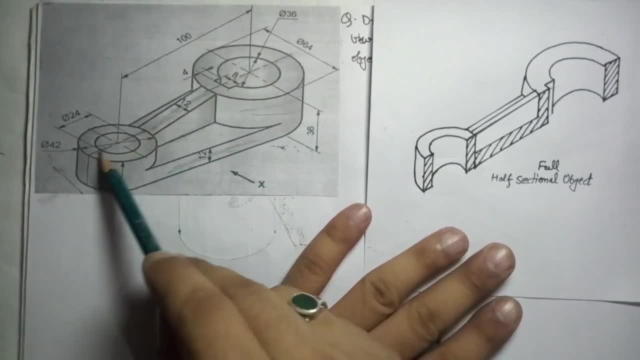 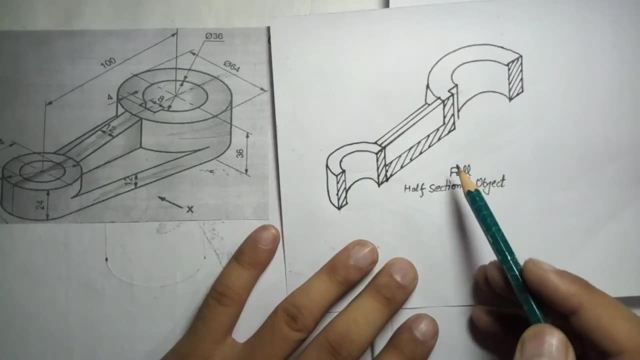 like this means we have to cut it from here, passing from here and then here. When we have to cut and remove this part, this is the remaining portion. In short, I can say you are going to draw the full sectional front view of this means this is the front view This question can. 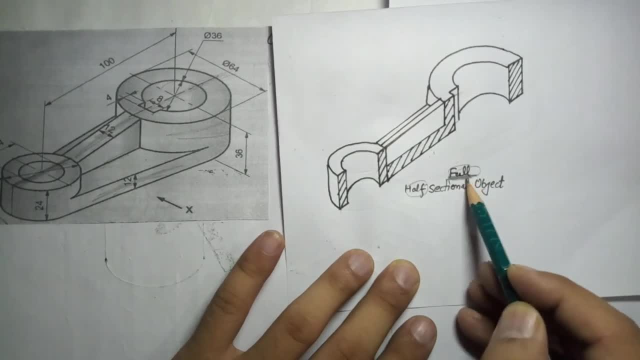 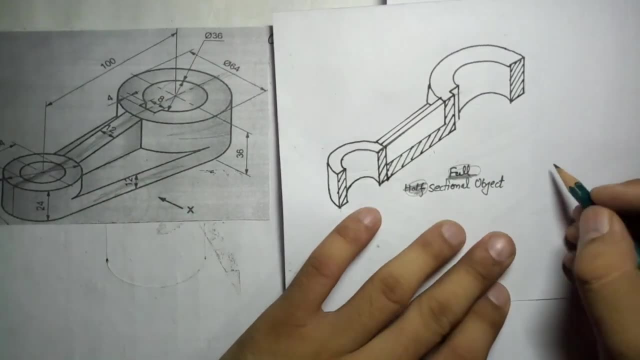 come for full or half, but we are solving for the full, so we are not solving for the half. Remember this. Now, first step: draw the normal orthographic projection. Now, what will be the normal orthographic projection? Here you can see a straight line and a cylinder. 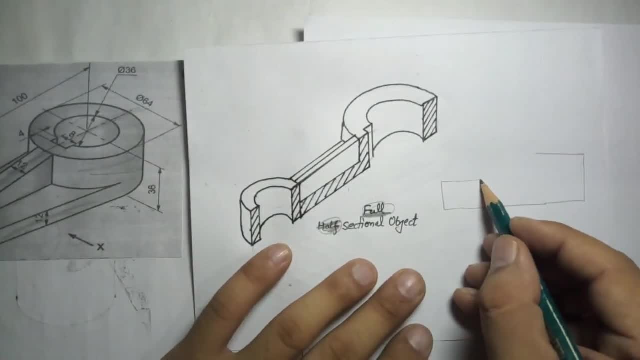 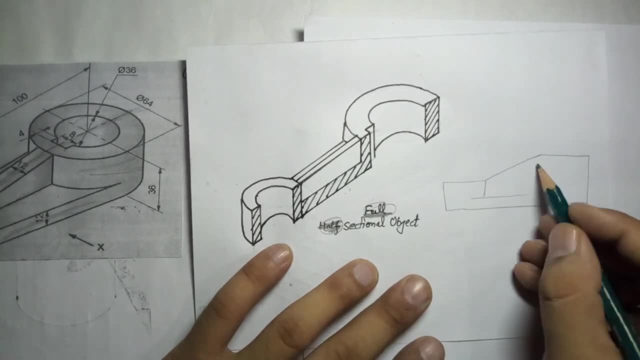 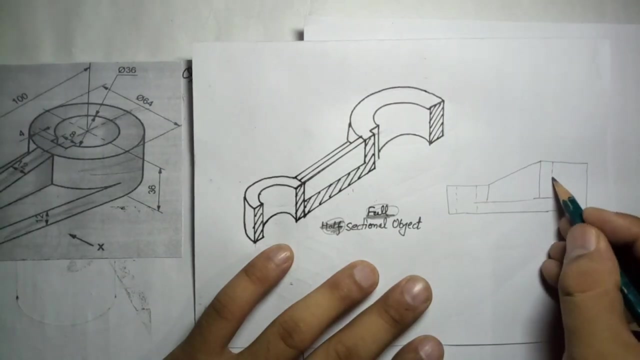 here also a cylinder. I have discussed all the orthographic views in the previous videos, so if you have any doubt in that, you just try to follow those videos and it will be more clear if you do practice according to those videos. So this is the normal front view. Depth is not given. that is why I am. 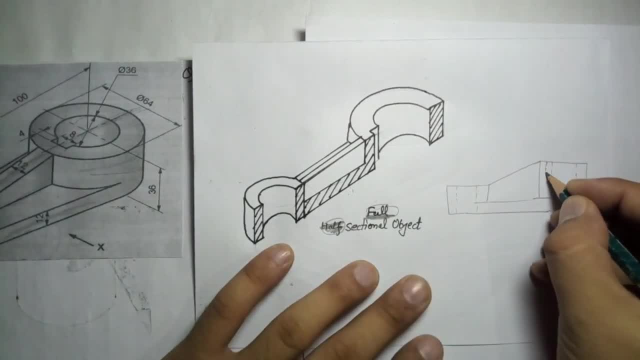 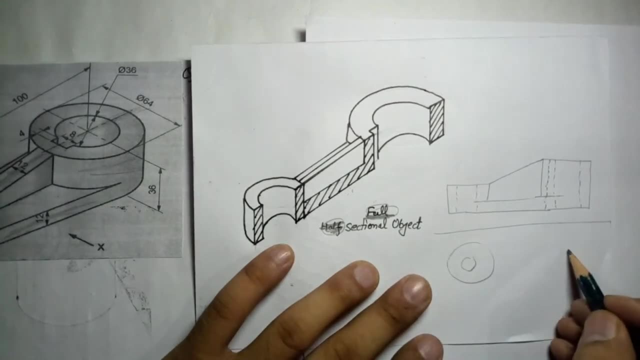 taking throughout. So there is one keyhole. so that is why it is having two hidden lines here in the front view. Now then the top view. This circle and this circle, Same here, a bigger circle and more bigger circle. It will. 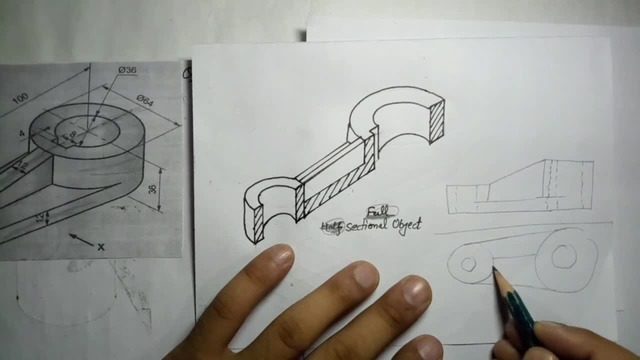 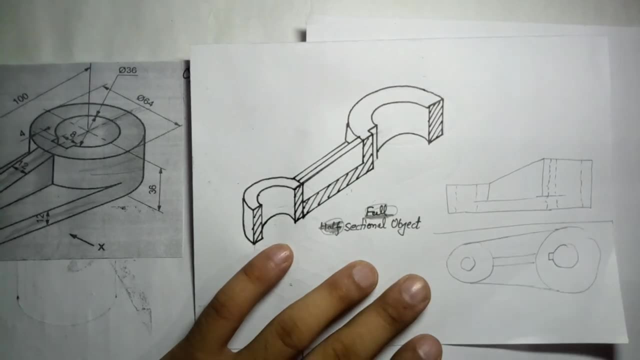 have the two tangents here and here, then a part is there, but here it is not only the circle, it is having the keyhole. So it will have this type of structure in the top view Right. So this is the front view and top view, Just to show you orthography I am making. 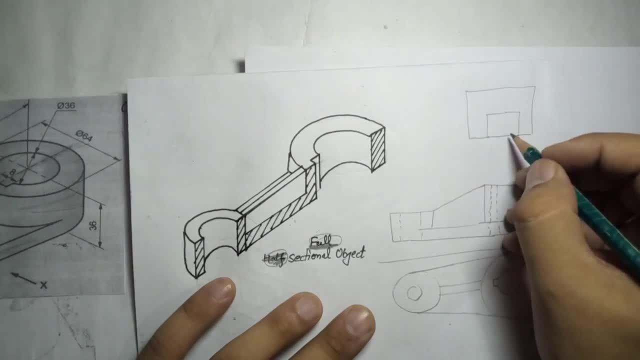 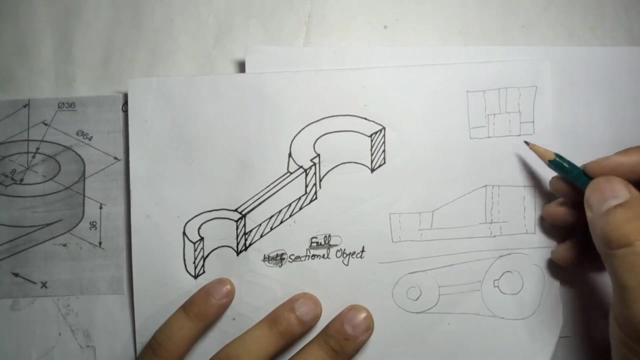 the side view. Just to improve your imagination, I am giving you the side view also. Please keep this on its own. So it depends where it will come as per the dimension. so you have to check. So this is the side view, Just to cross check. you draw the side view and 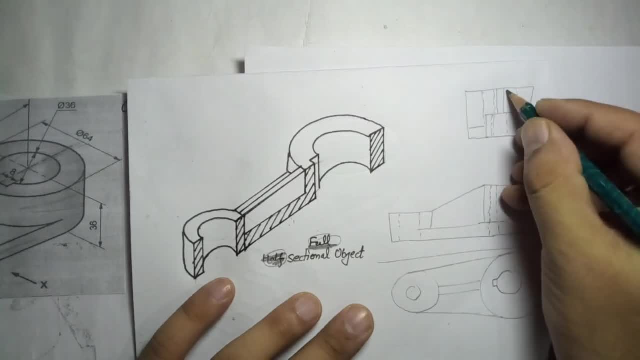 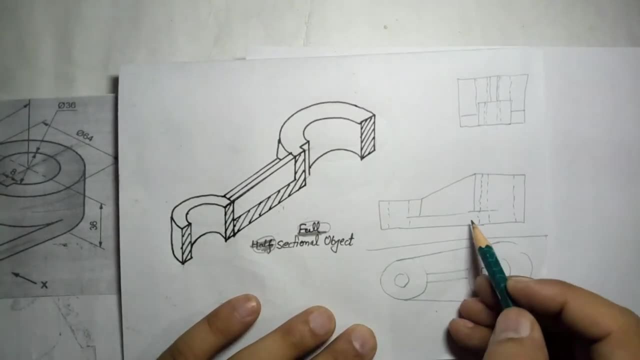 try to see Here. it will have one more hidden line for the keyhole. Okay, So try to compare your diagram. Now my main focus is on sectional view. So first step, we have done normal orthography. Then you have to convert the hidden line into object line. So when you cut and 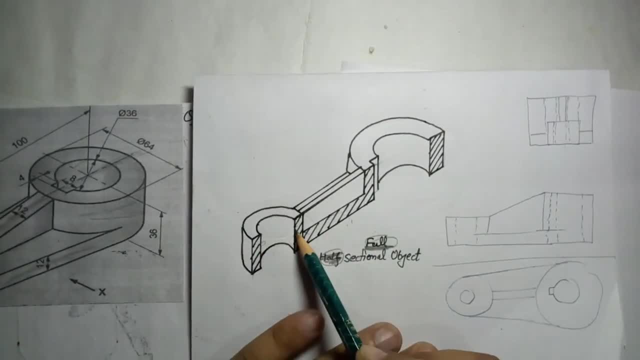 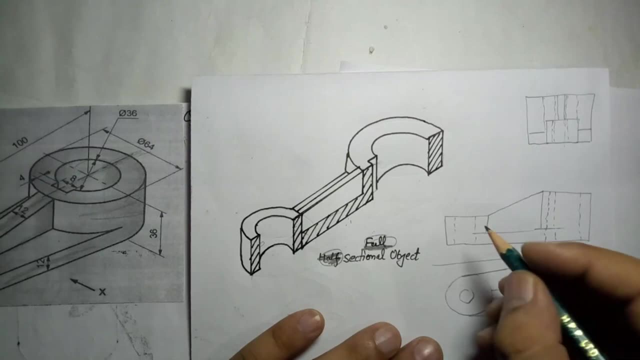 remove this part. this is the object. So it means these edges of the object which was not visible, but now they are visible. That is the meaning of second step: convert the hidden line into object line, which are coming under sectioning. So this is coming under. 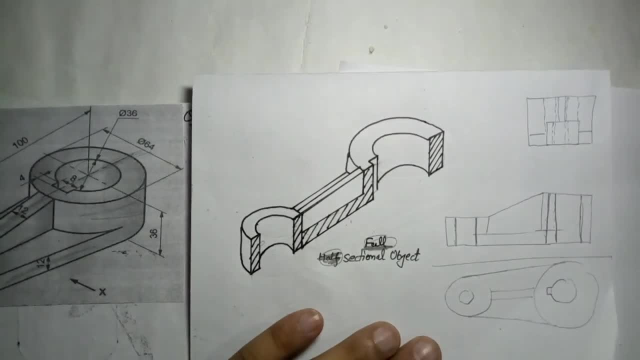 sectioning and this keyhole. it will also be dark now. Now this base, it will be present in the object or might not be present. It depends how you are taking the objects. Let's say, we are not taking this means in this object, you are taking this surface, This surface. 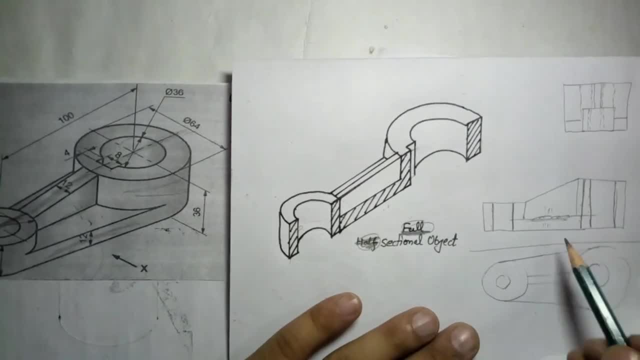 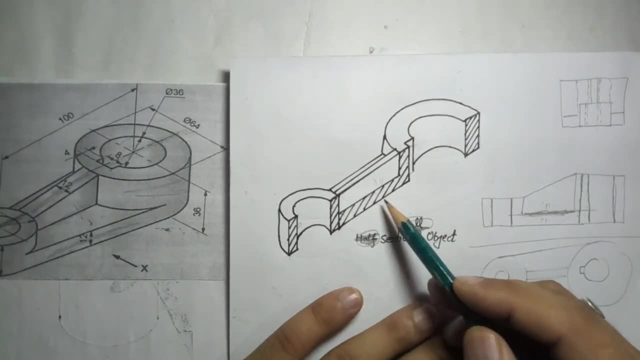 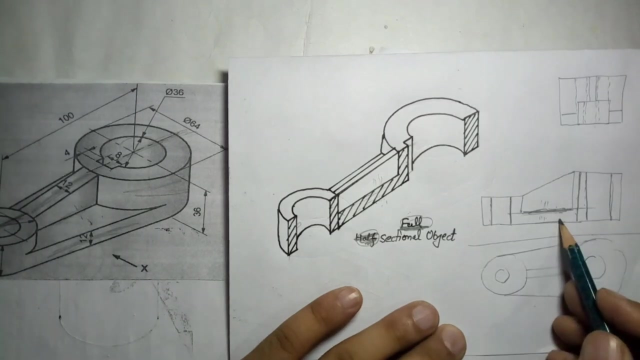 and this one as the same single surface. But here I have taken this base because I'm taking this surface and the rib as the separate one. So that is why in my diagram it will be present this surface and this one. So we have to draw this as a dark line. Now we have 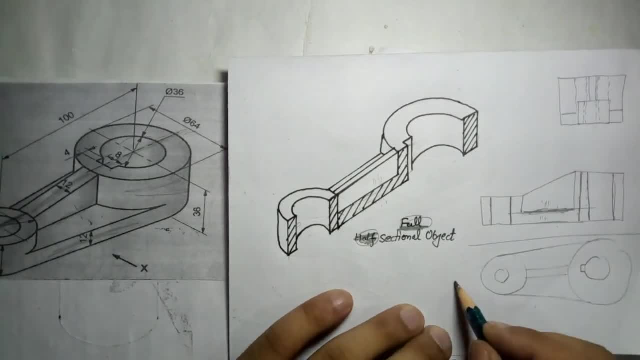 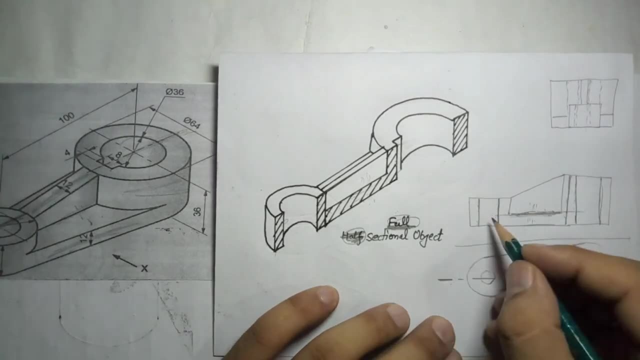 converted all the hidden lines into object lines. Now we will draw in the top view the section line. This section line will come in the top view just to show you the position from where we are cutting the object. And now we have to do the hatching. So we are. 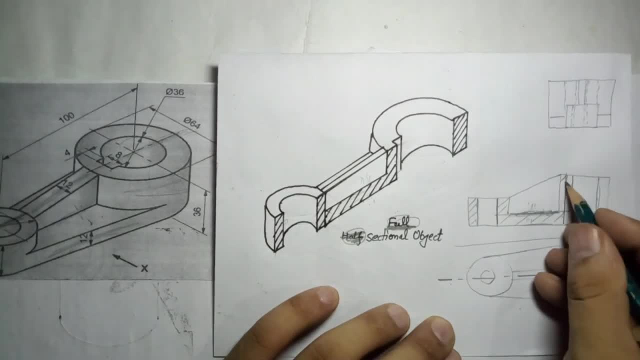 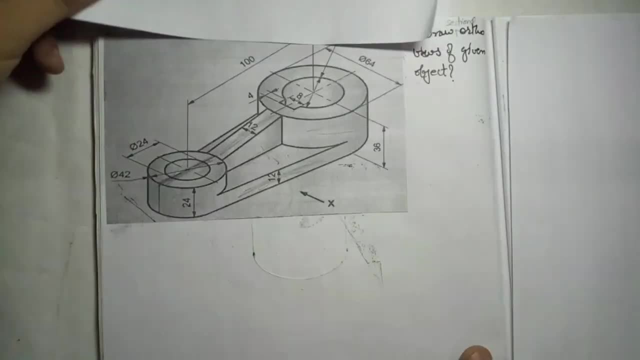 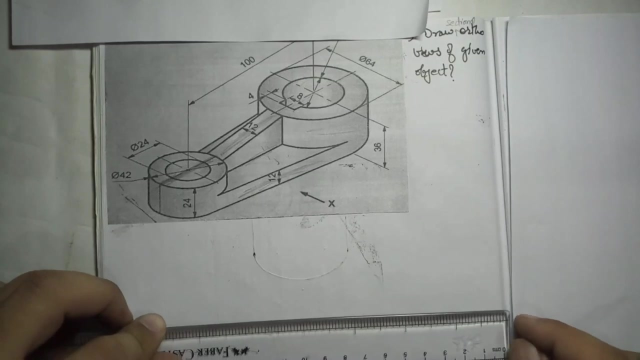 going to do the hatching. So this is the area where blade is making the contact with the object. So we have to do the hatching on that area as per the rules. So this view we are going to make on the sheet. Now I will draw this view, taking the dimension from here. 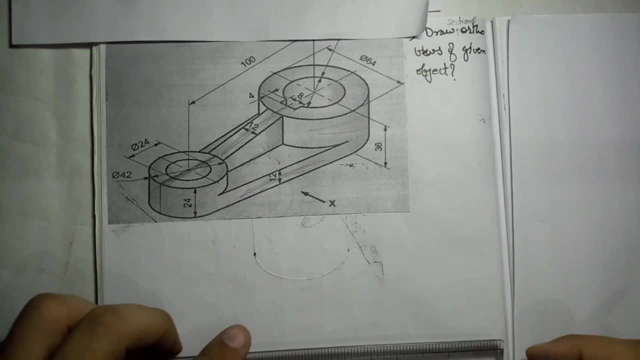 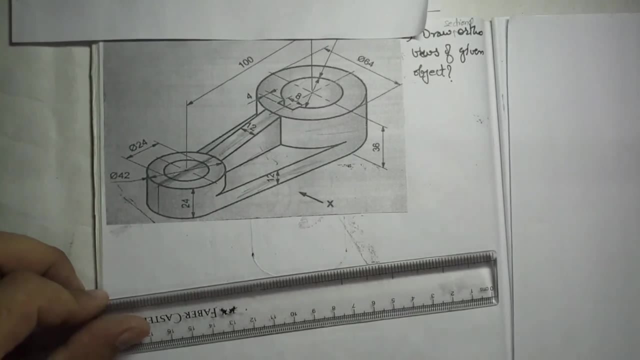 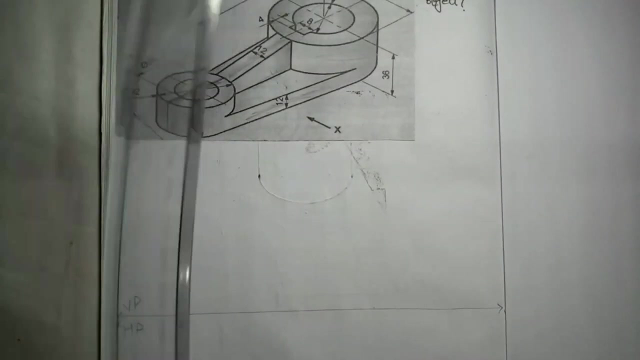 And the total 64 is there. So I need more space in the top view. Now I will draw the xy line. We are solving it in first quadrant, So vp above, hp below. Now, after that, what I have to do, we have to take two grid point gap here. Done with that, Now the total dimension. 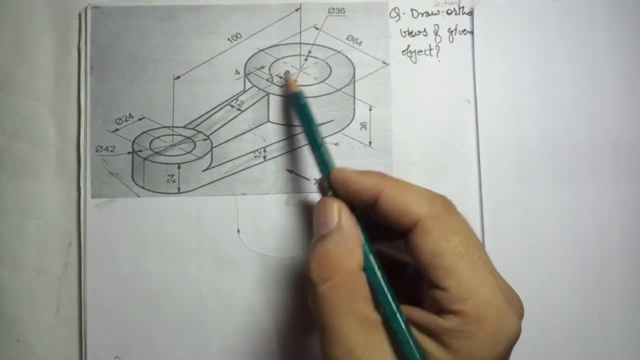 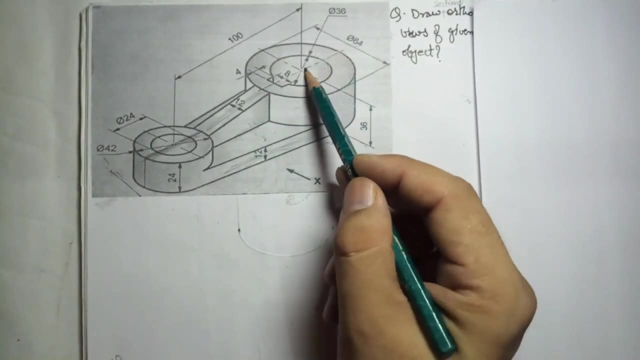 how to calculate total dimension from this mid to this. it is given 100, 100 plus radius. of this 64, half 32.. So 100 plus 32,, 132,, 132, then again half of this. This is diameter. 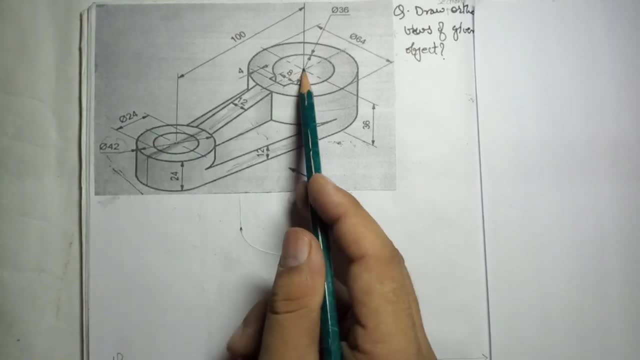 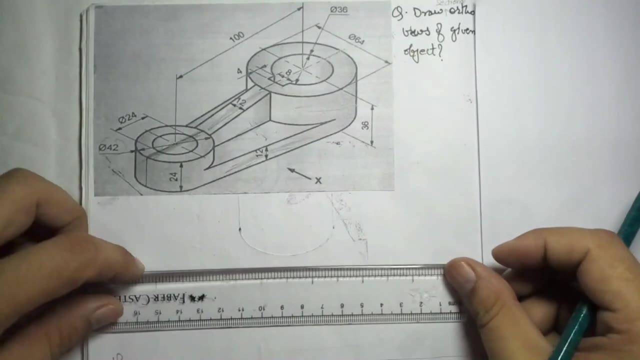 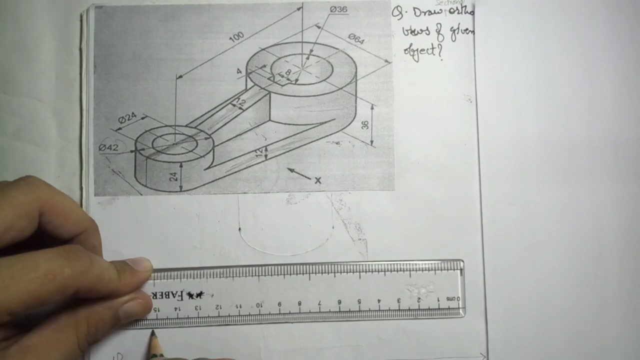 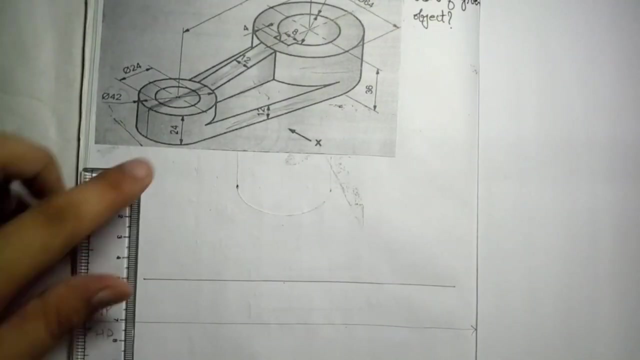 42 after 21.. gives 100 plus 32,, 132 plus 21,, 153.. So total length of this is 153. So I am taking it 153.. Now, after that, what we have to do, we have to take the height 24.. So from this, I am taking: 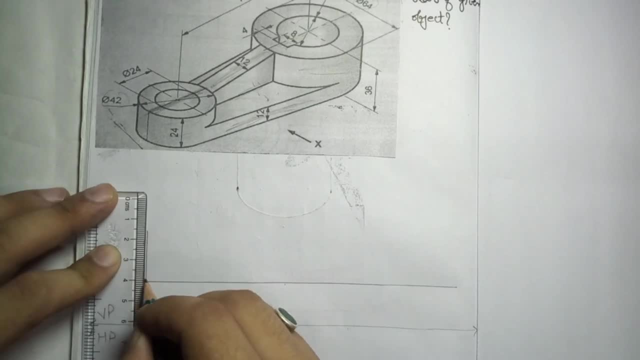 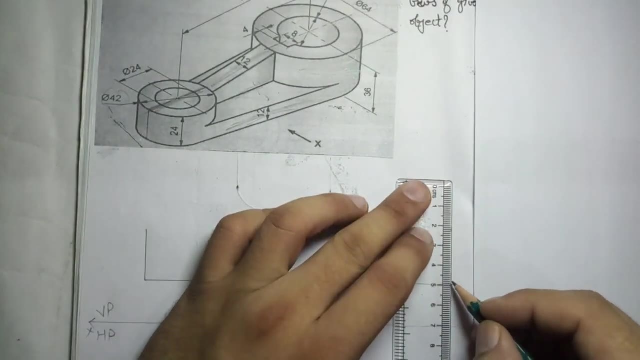 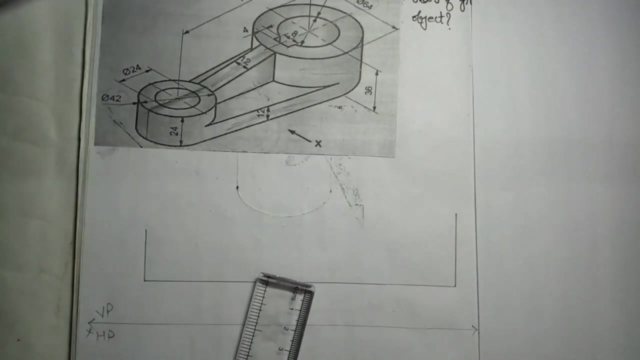 height 24.. You have to draw very quickly… Okay- the diagram, because in exam you will have only 10 to 15 minutes. so this is height 36. so on this side you have to take 36 right now. after that you can see here i am taking the help. 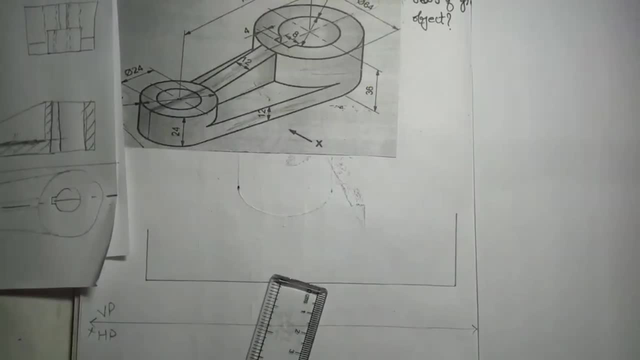 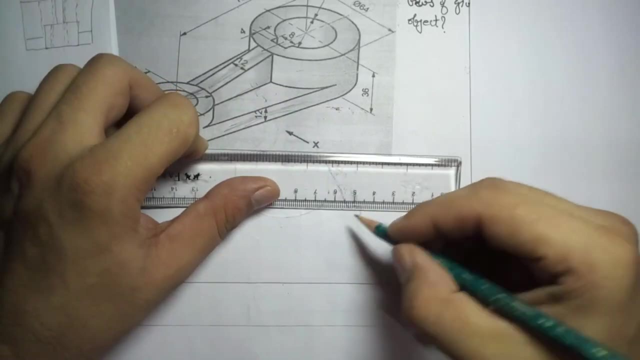 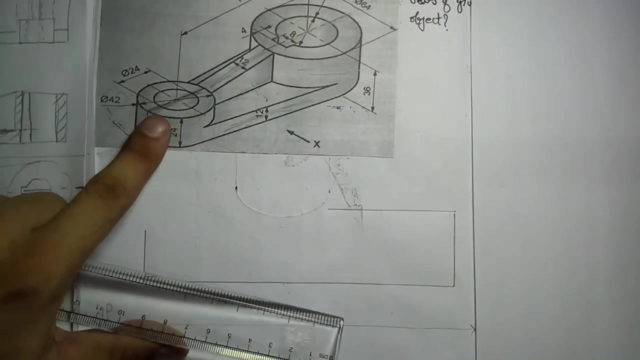 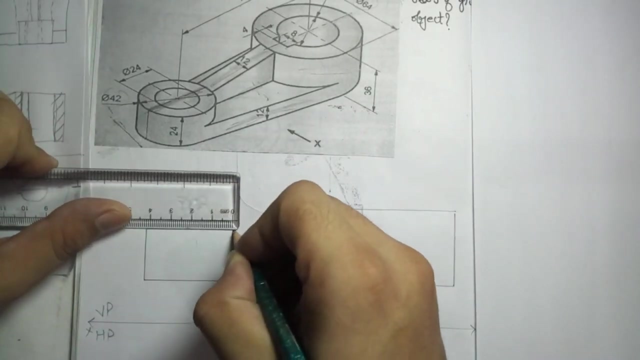 of this diagram with the dimensions. now it is having diameter that is 64, so i'll directly take 64. very quickly, take the dimensions, try to draw exact horizontal line. done with this, then this smaller. it is having 42, so i'll take exactly horizontal 42 now. after that i have to join them. 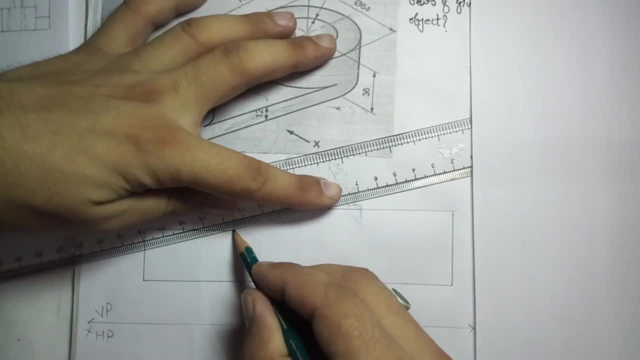 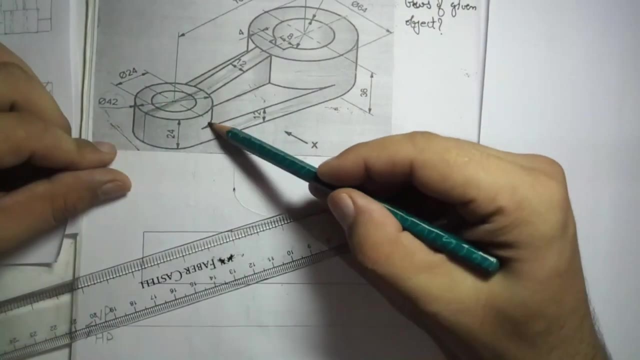 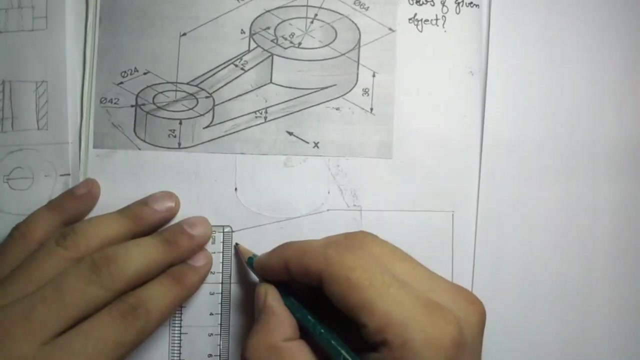 for the rib done with this now. after that it is having this part. now i'm going for this part. this is 12, it is 24, so this is 12. let's do the practice of calculating the dimensions in exam in questions. they will not give you all the dimensions directly. you have to do calculation. 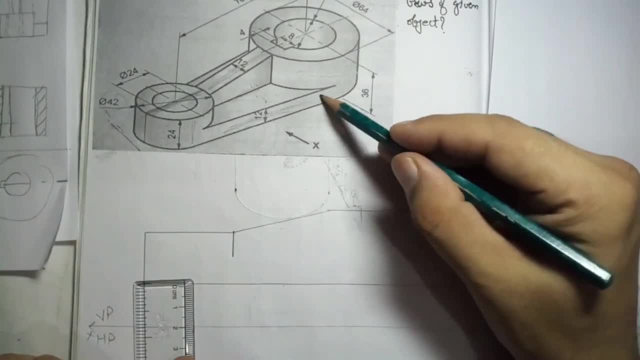 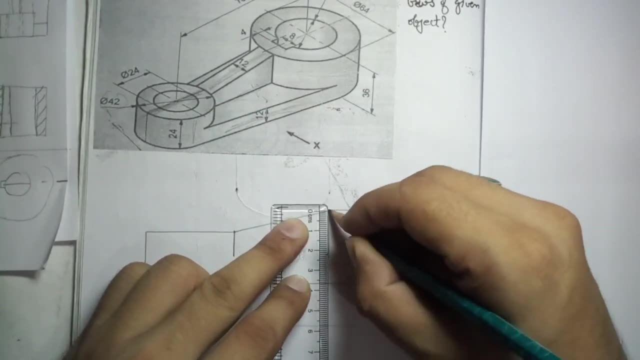 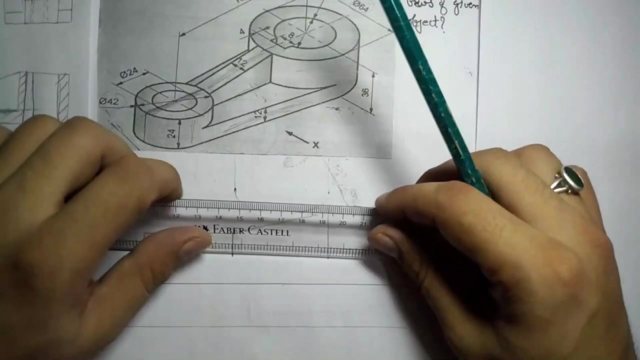 now this is 12. here it was 36 minus 12, so this is 24. so from this i'm taking 24 done after that. if you are doing the question like this means you are taking the two separate surfaces. so i'm making this line, i'm joining. 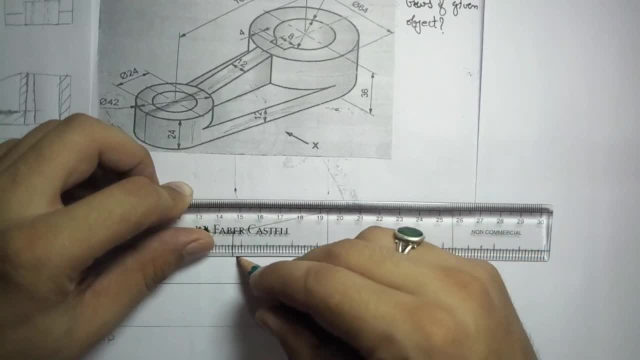 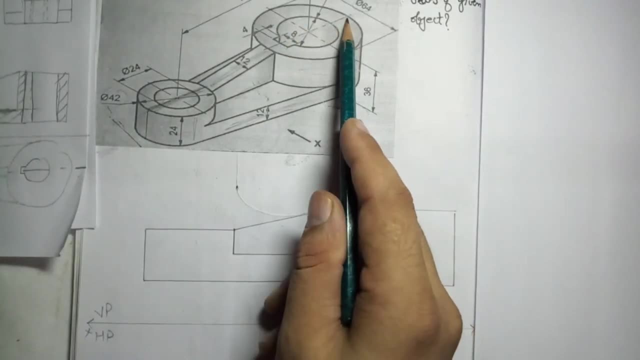 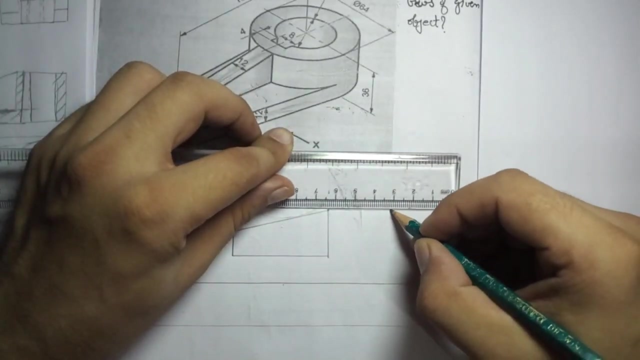 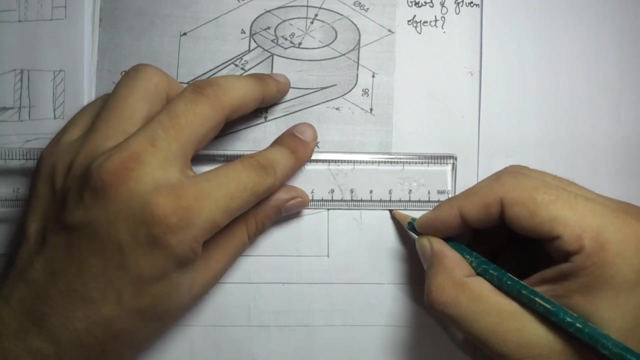 this, taking rib as the separate object done with this. now there is the internal diameter. what is that internal diameter? that is 36, so i have marked the center point. so this is 64, that is 32, so you got this center point. now about the center point: it is internal diameter, 36, so 36 means. 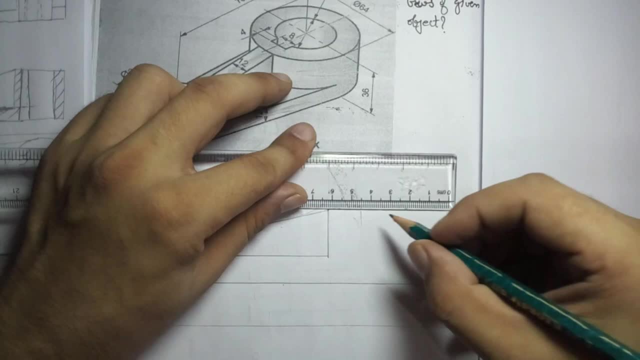 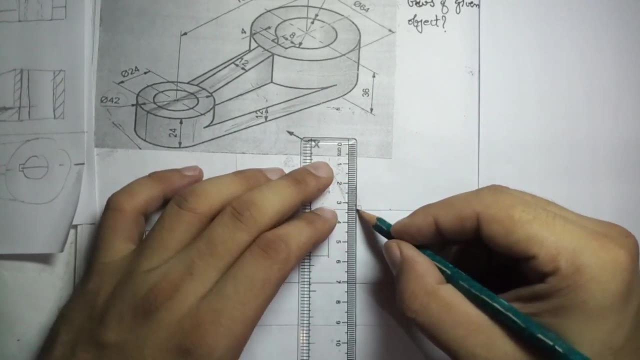 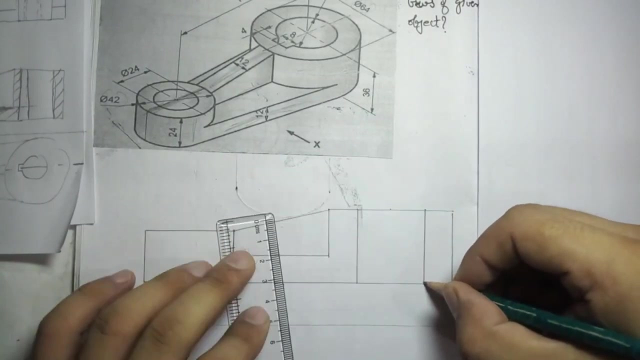 18, 18 both side, 10, 8 on this side, 10, 8 on this side. without sectional front view, it will have the object line. sorry, hidden line here, but sectional view. it will have the object line. done with this now. after that there is a keyhole. 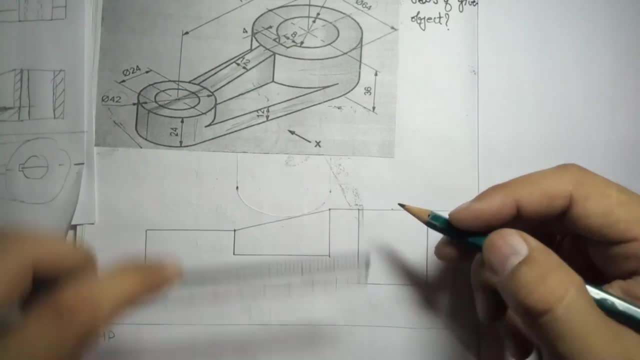 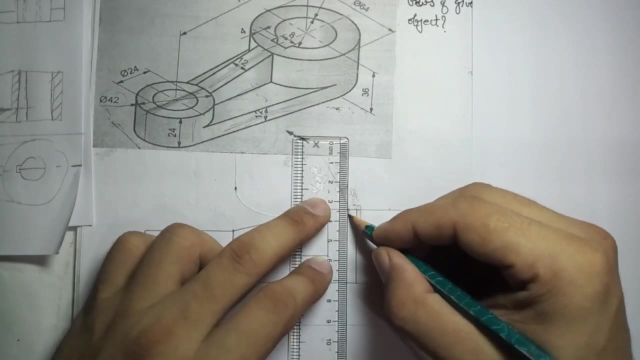 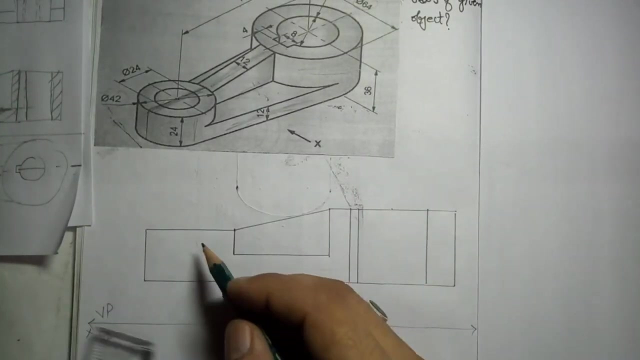 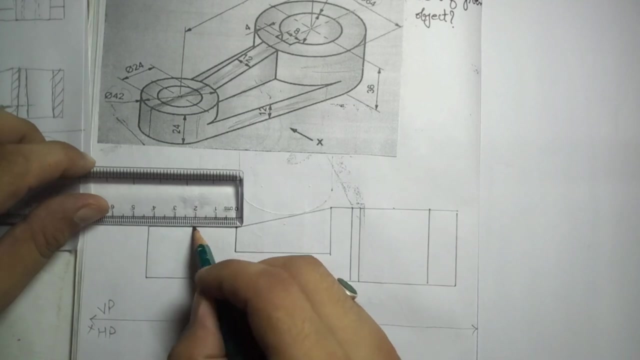 from this. it is four only, so i'll take directly from this point. i'll take four directly and mark this keyhole. done with this. i'm taking the holes throughout right same on the side at the mid it is having internal diameter 40, 24. so i'll take 42, mid, 21. after that, after 21, it is 24. so 12 on this side, 12 on this side. 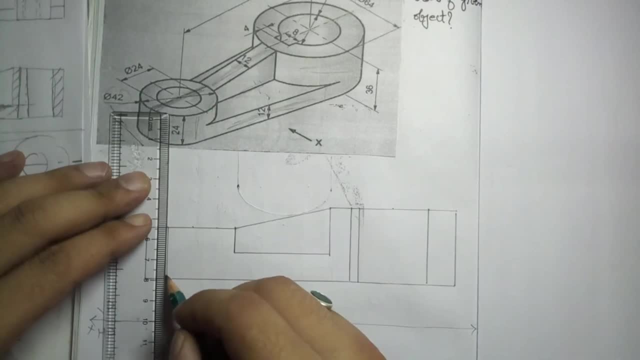 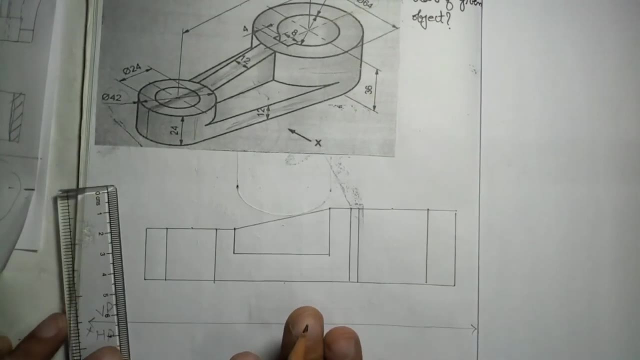 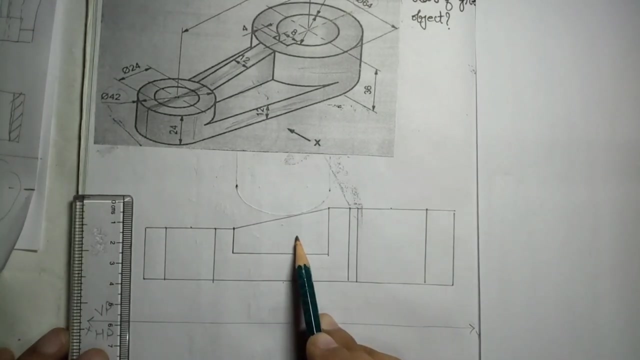 while drawing, learn how to calculate the dimensions very quickly. you should draw this. so this is the front view. now we have to draw the hatching now where the blade will touch in this area, in this area and in this area. no need to make the hatching here. this is rib part, so i have told. 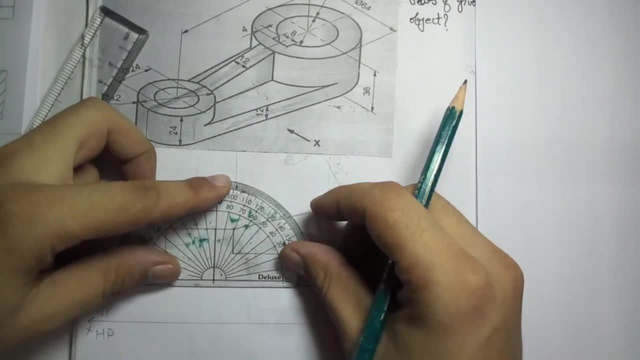 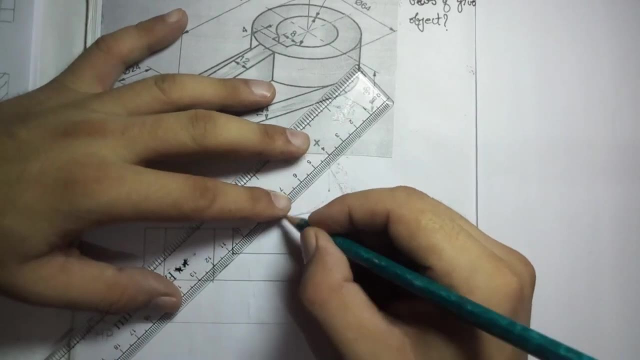 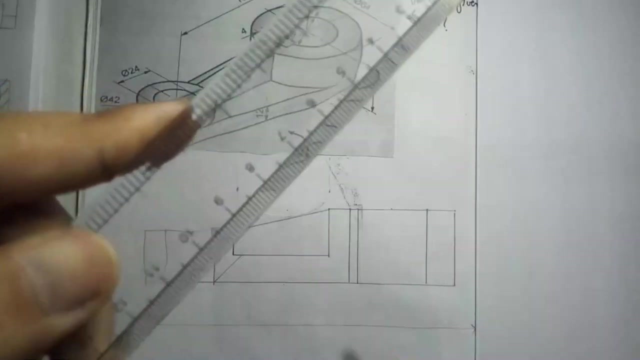 you how to do the hatching from any corner of the drawing. assume the baseline horizontal, take the 45 angle for the reference line, mark this point. okay, so we draw this. now i have told you. take the help of this, the drawn, this line. if you can see this line, which is already there, it put it on the drawn. 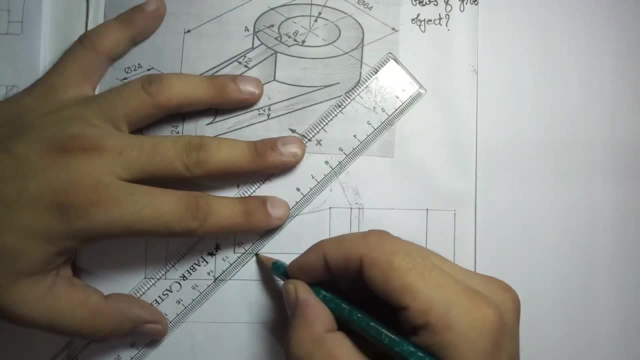 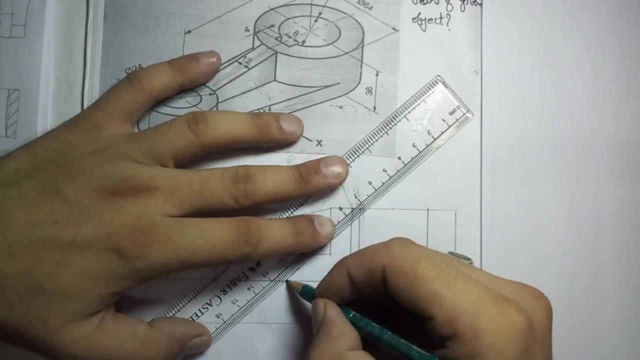 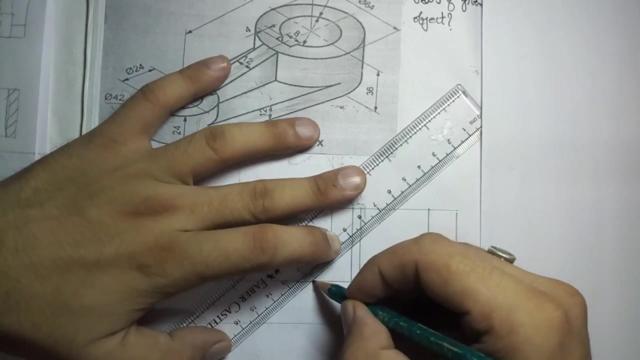 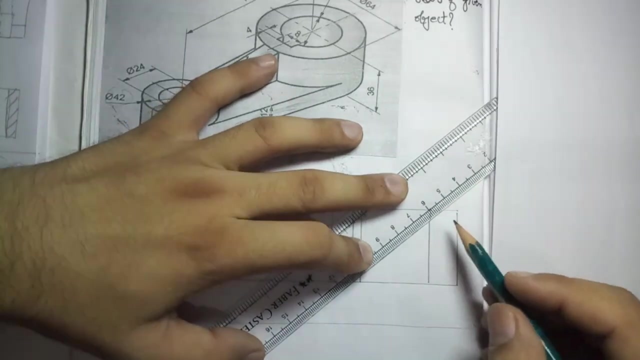 line, then give the gap continuously. you can take the hatch lines in every scale. if you focus on this area, it will be in the range of two to five mm. no need to worry about the gap. it will come exactly parallel and constant gap between two to five mm. remember that: continuous and the same. 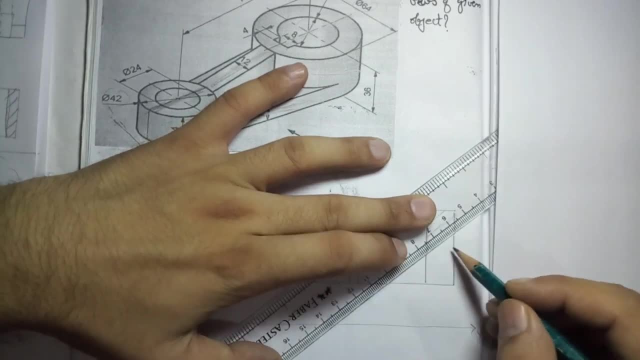 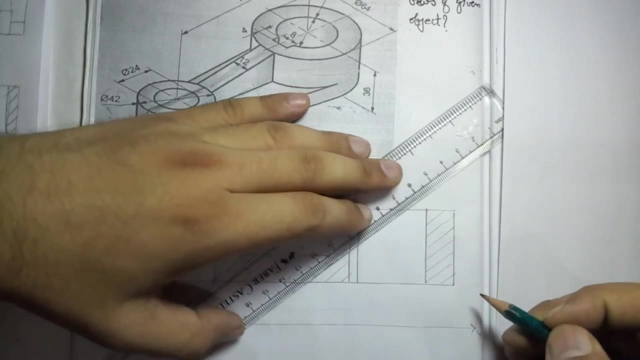 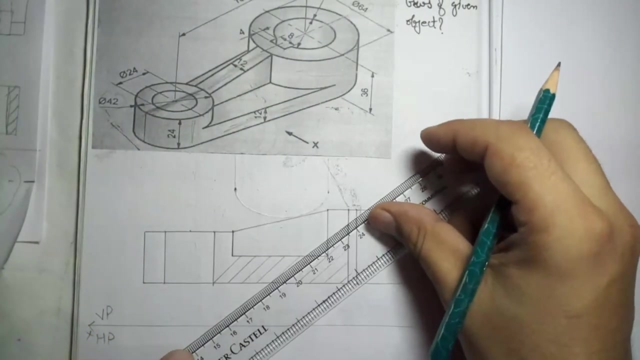 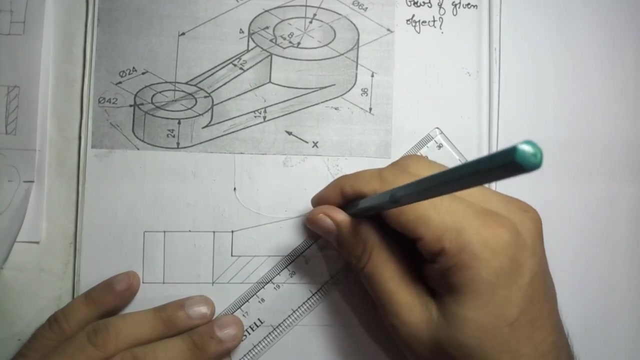 throughout the diagram, continuous line must go for hatching like this same. you can follow on this side also very quickly. we have to complete the diagram. please try to make the diagram within 10 minutes so that in exam you can solve the same complete diagram within 10 minutes. 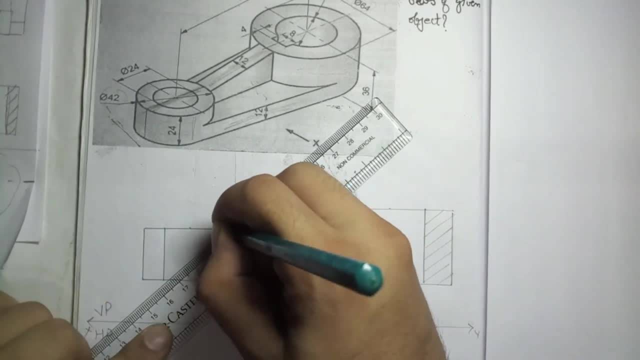 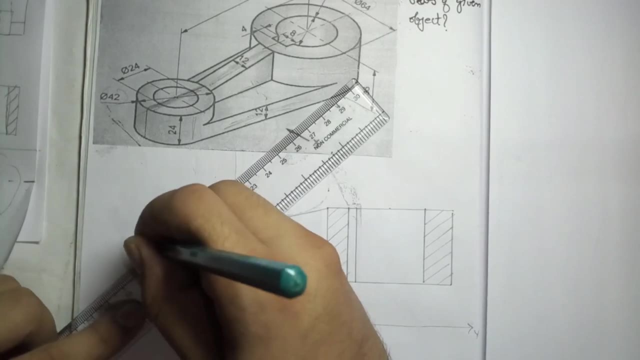 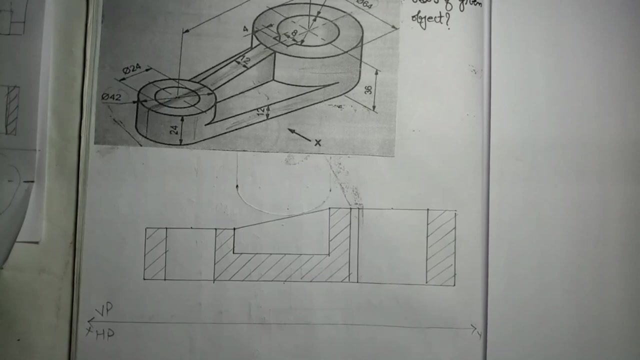 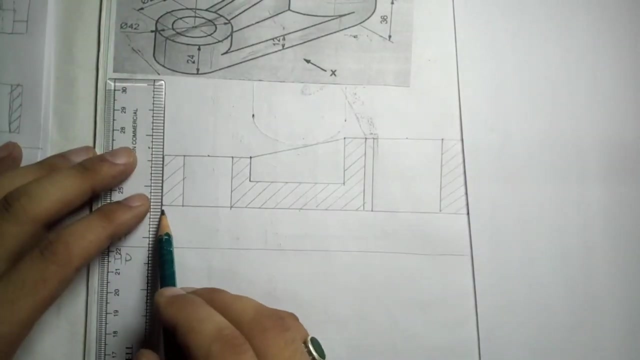 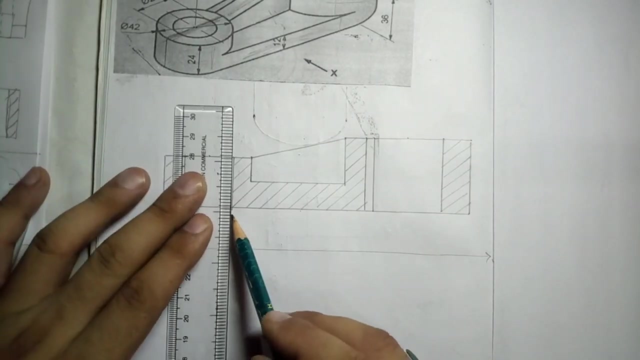 right. so this is the sectional front view. now we have to make the top view. i have told you to make the top view. take the projection lines, be quick, take the projection lines downward from each and every part of the object. actually, i have follow those key rules in the free hand: catch first. i haven't done the normal. 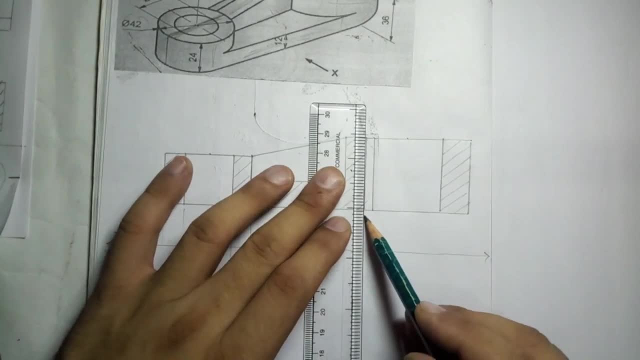 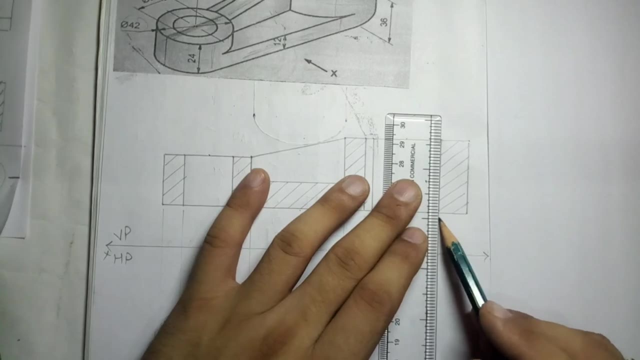 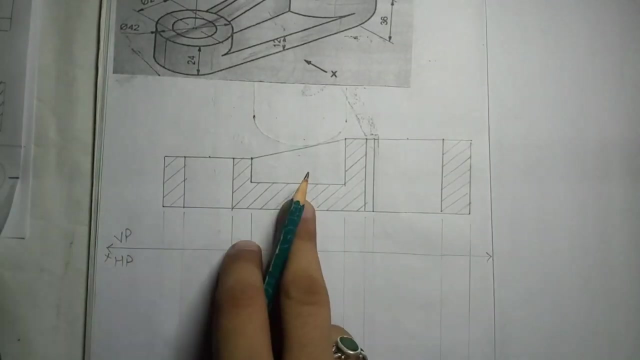 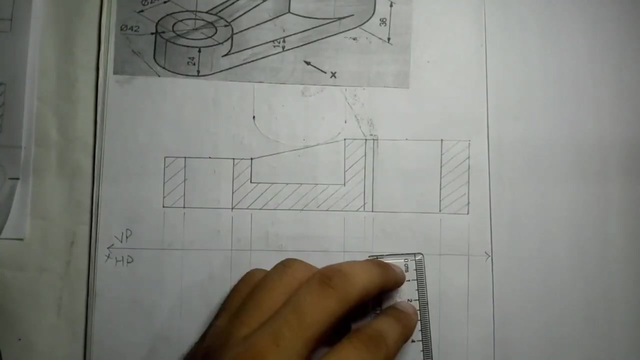 that we talked you after that have wrong the i have a opportunity having language object � means now the diameter is sixteen and then i can complete the diagram線 выпуск rating に so i have to take the dimension so that it should come so if i leave two grid point here after that 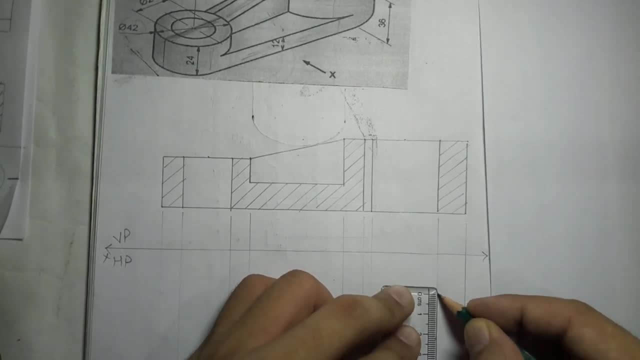 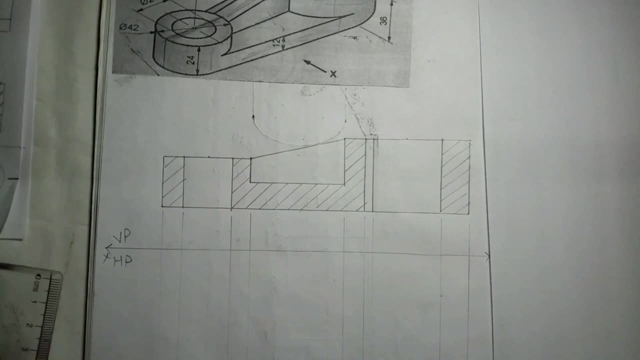 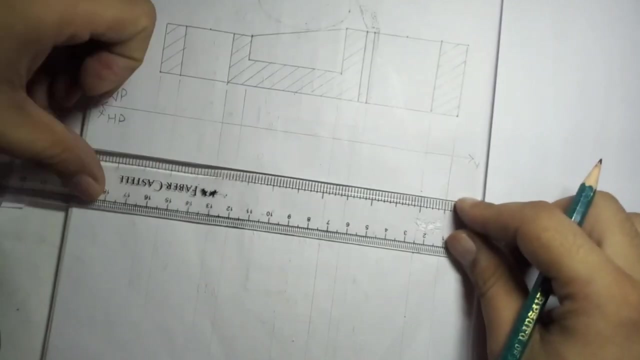 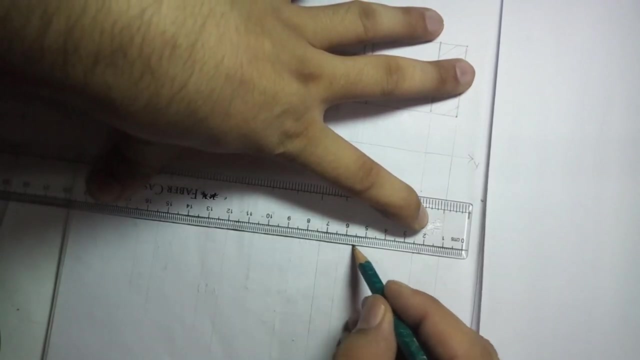 i have to take 64 diameter, so i will directly mark 32 for the midpoint of the circle and then 64 as the diameter. so this is my question. here it will come like this: now i can make the horizontal center line, just to make it easy, while drawing the circles right after that. you can, if you. 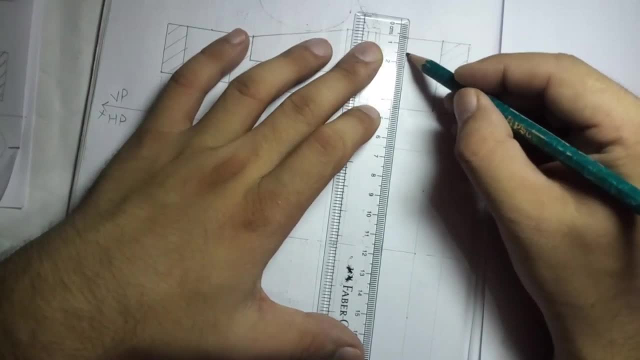 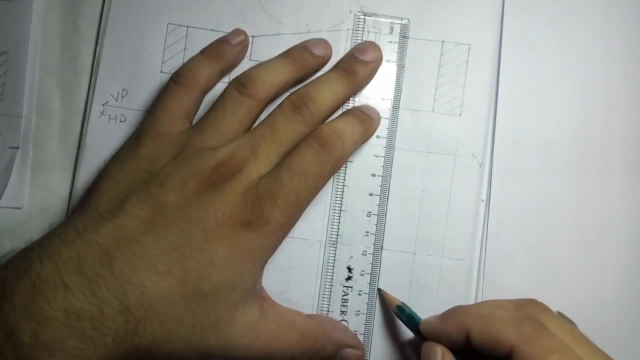 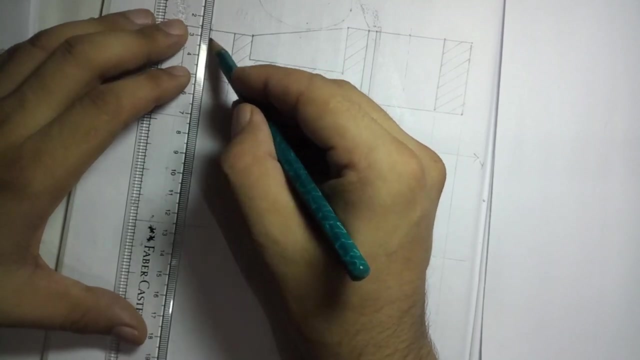 want, you can take the middle line, center line from front to top, also one long, one short line. proper formation of center line. for for this also we have marked the center point at the top so you can take directly the projection line. it will help you in top view. 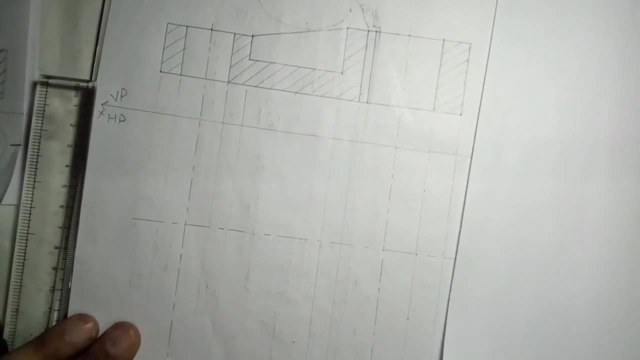 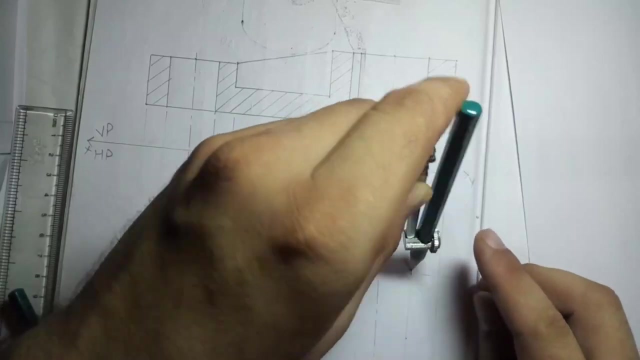 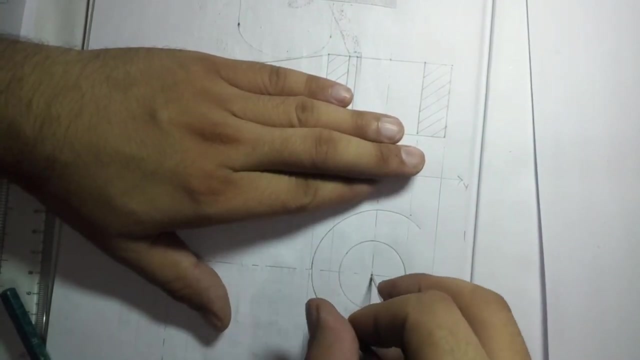 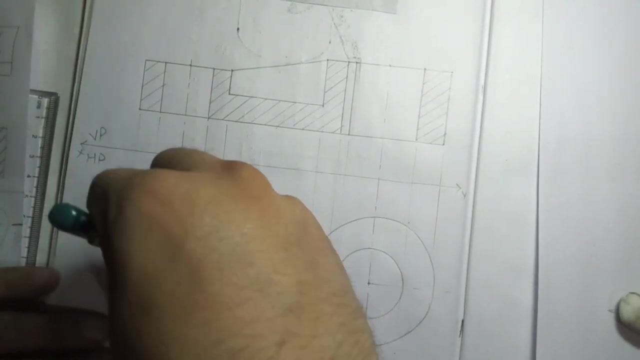 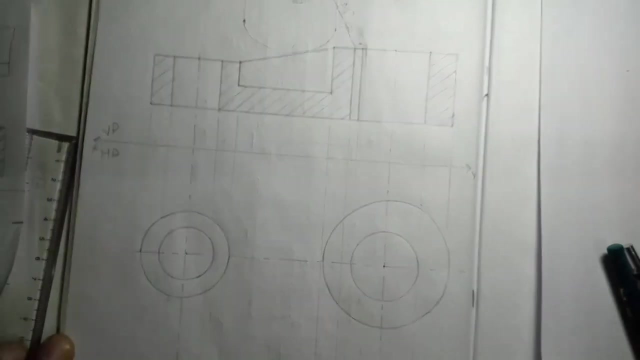 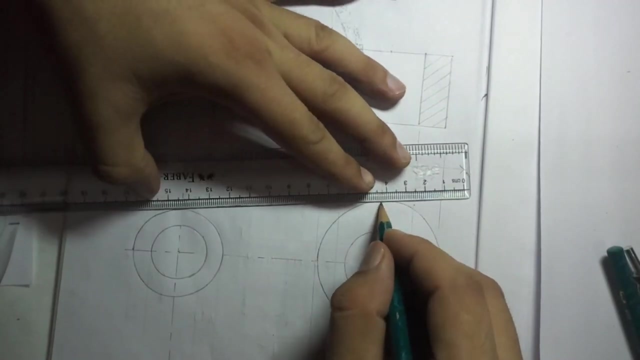 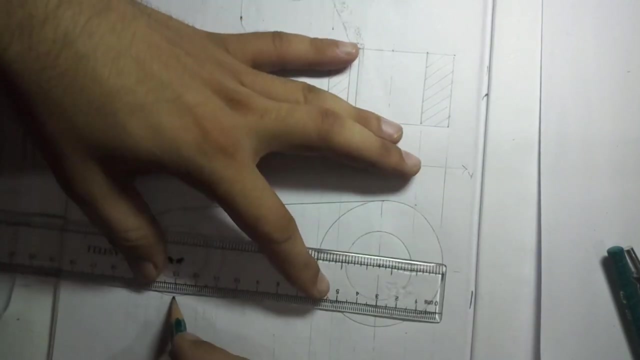 after that i will erase the extra lines. now we have to start with the circles. so first the internal circle. so i have done the required circle in the top view. now i have to make the tangent just join it. put the scale and join it, just a tangent on the tangent line. 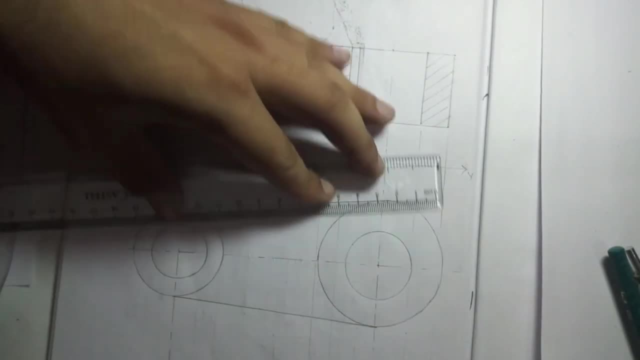 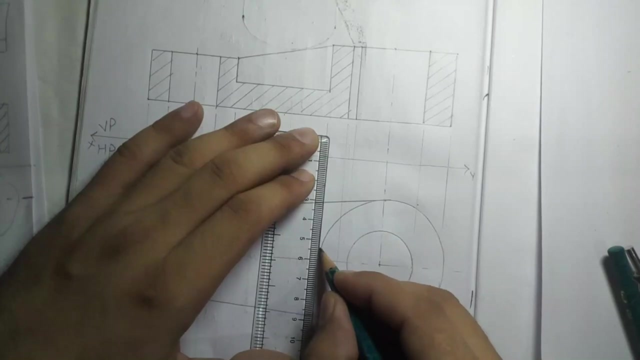 make two circles wherever it is just joining. just draw that right now. inside there is a rib of 12. so on this side. so from this, 6, 6 both side. so i will mark 6 on this side and 6 on this side, two straight lines. 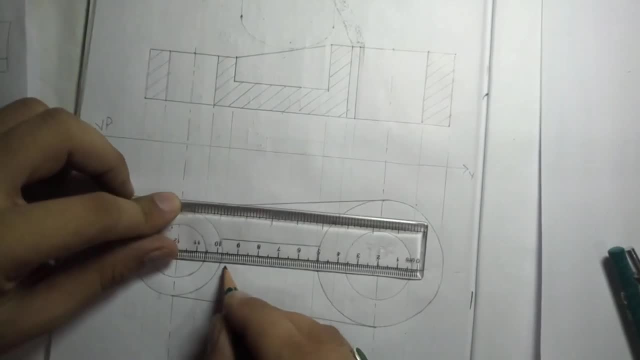 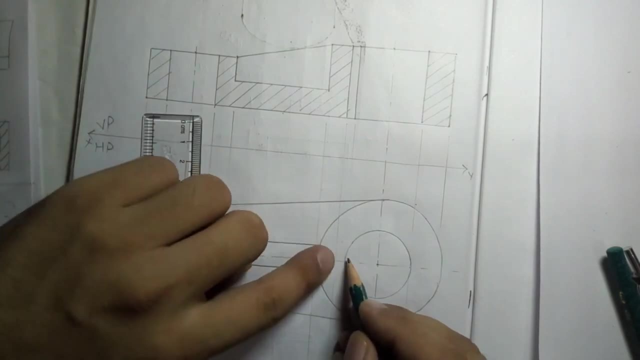 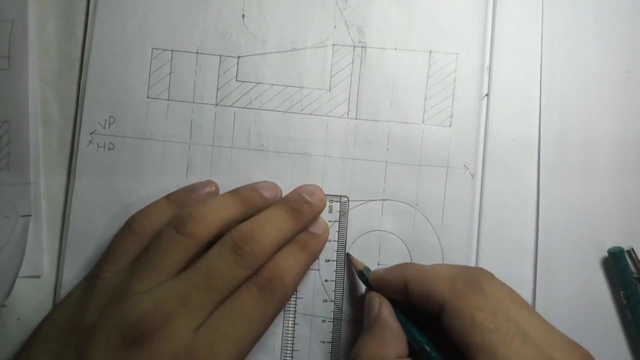 for the rib part like this. now here is one keyhole. keyhole is having a value of this projection right, so we will follow the same. this is what: 8. so 8 means 4, 4, both side. so from this side i have to mark 8, 4, 4. 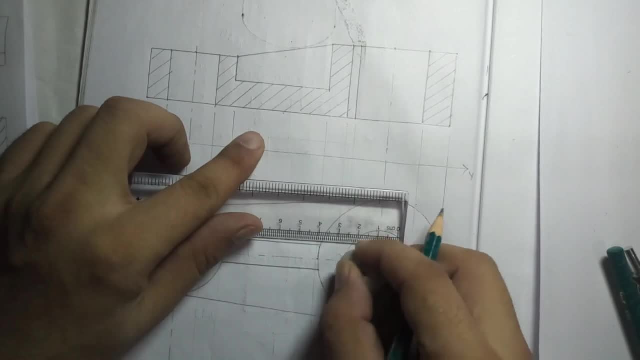 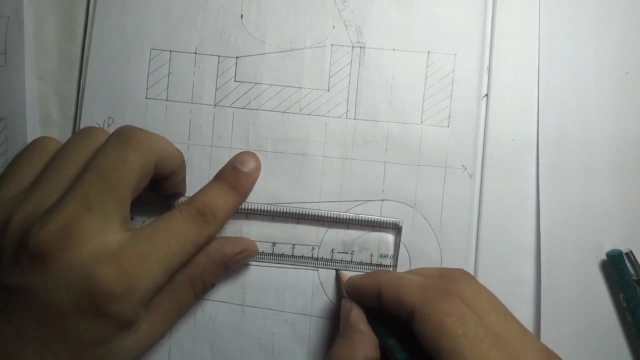 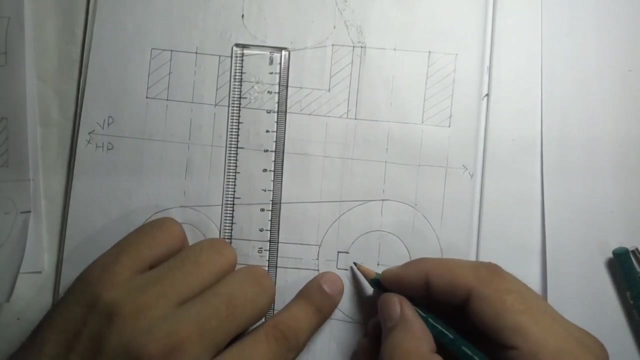 this is the. now i can erase this part of circle to make the keyhole. now i will make the straight part, this straight part, this sharpen pencil after few lines, otherwise it will start making the thick lines, like i have done this here. so this is the mistake. 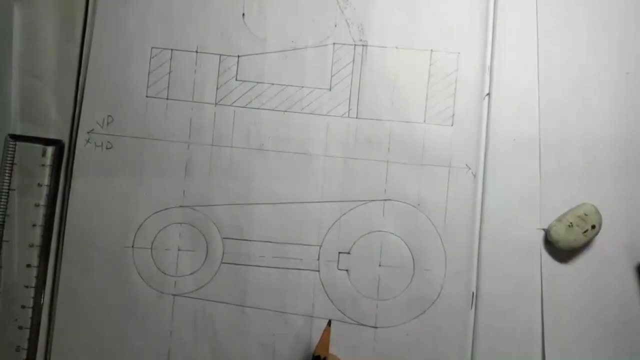 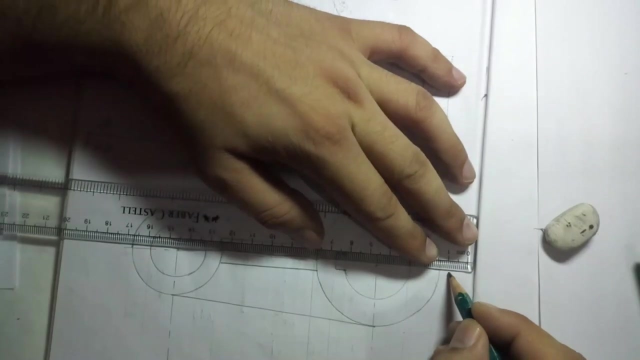 sharpen your line after making few lines. this is the front view and top view. now, in the top view there must be a section line, so i have drawn the center line. i will convert the same center line into section line. how? only the outermost edge is dark. 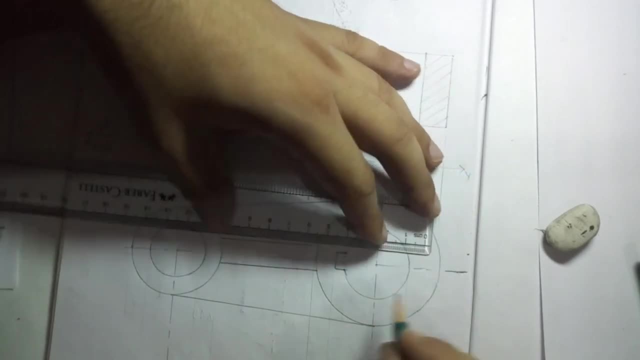 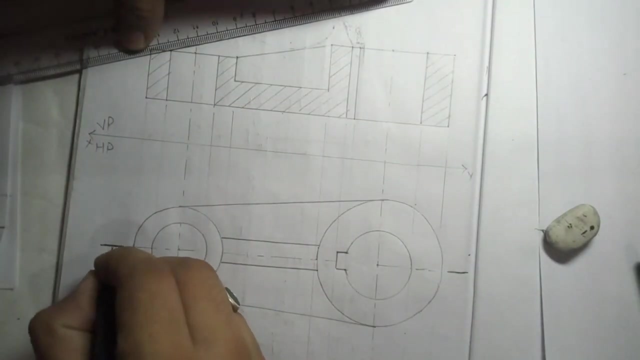 i have told you what is the section line. it will have the same shape of center line, but only outermost edge is dark. so that is why i have made this and this thick. now it becomes section line. we are cutting the object from here. now i will do the dimensioning.